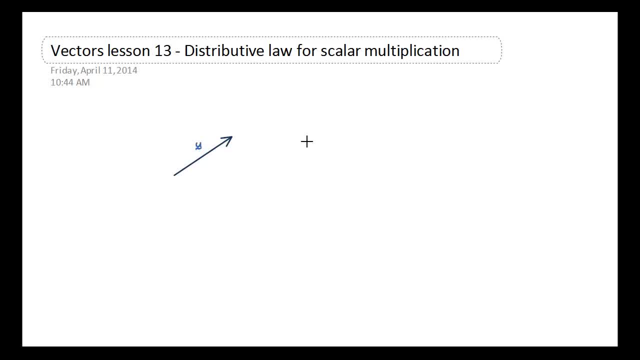 a vector here that I'm going to call vector u. if I was going to draw a vector which is 3 times u, then what I have to do is basically copy the same vector again but make it 3 times as long. So I'll make it 3 times as long in the same direction. Okay, so this vector here would: 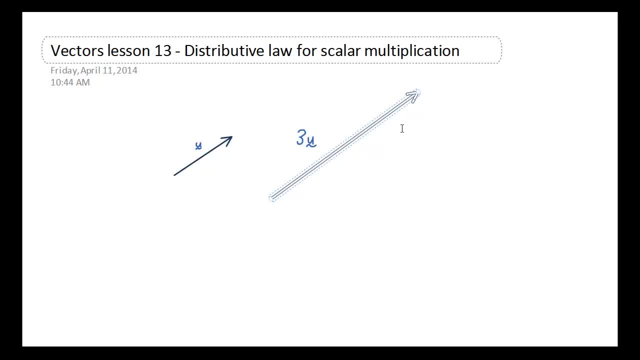 have the same bearing as this vector, but it is 3 times as long. Okay, so now let's talk about the distributive law. What is the distributive law? So let's imagine that vector u is written as the sum of two other vectors. 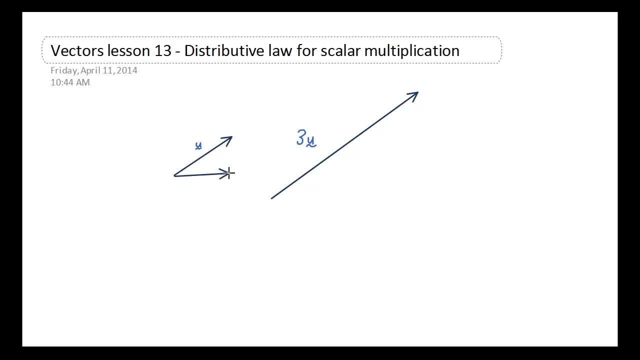 Now they can be in any direction, but just to make it simpler, I'm going to make them horizontal and vertical. So vector u is now the sum of two vectors. So I'm going to call this vector. you can call them anything, but I'm just going to call them a and b, Vector a and vector b. 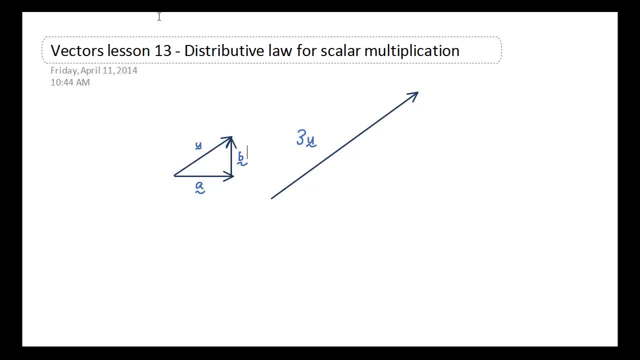 Now, if I make u 3 times as long, then what's going to happen is that a and b will also be 3 times as long. using the rule for similar triangles. Alright, so using the rule for similar triangles. 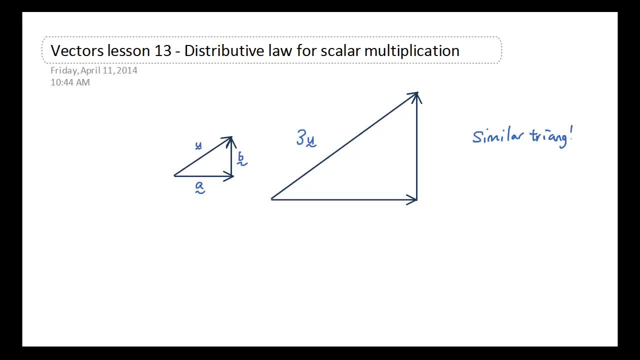 triangles. this side is going to be 3a and this side is going to be 3b, So basically, all three sides will need to increase by the same scale factor if you want this shape to remain similar to that shape. Okay, so bringing this back to scalar multiplication now. if you imagine u vector, u is multiplied. 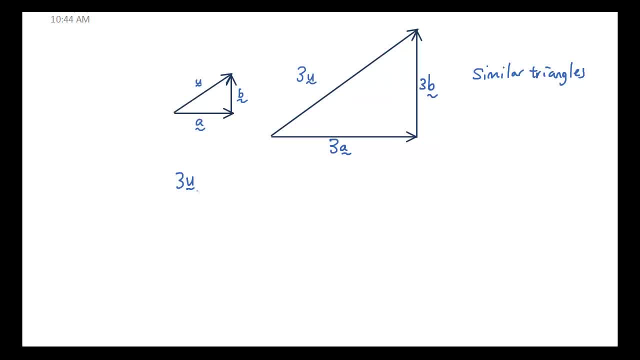 by a scale factor of 3, so 3u. instead of writing that, we can write it as 3 bracket a plus b, Right? so 3 vector u equals 3 bracket a plus b, Because u is equal to vector a plus vector b, as shown here. 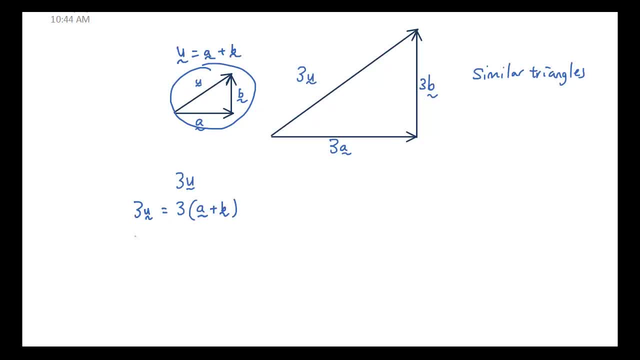 Right now 3 bracket, a plus b, as shown to you in this diagram. So u is the same as 3a plus 3b, Because 3u- this thing here is the same as. okay, I'm just going to write a plus b here. 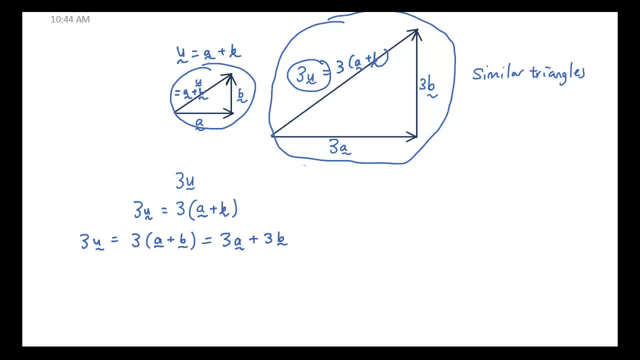 So 3u is the same as 3a plus b. so 3a plus b is the same as 3a plus 3b. So therefore, what we have just proven to you just then is called the distributive law. If you remember, in algebra we have something like this: a bracket b plus c can be rewritten. 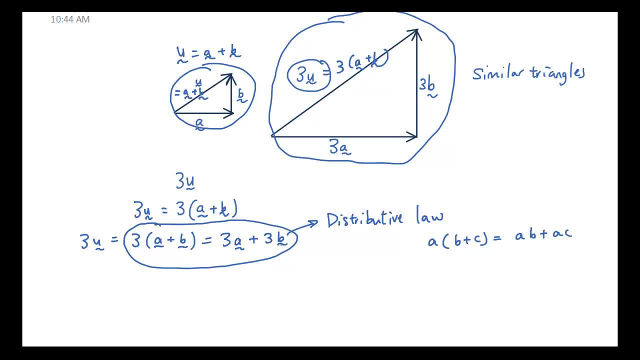 as ab plus ac. And now we have shown to you the same thing with vectors, right? Because instead of 3 we could multiply this by any scale factor. So instead of writing 3,, I could write instead of 3, just any number. 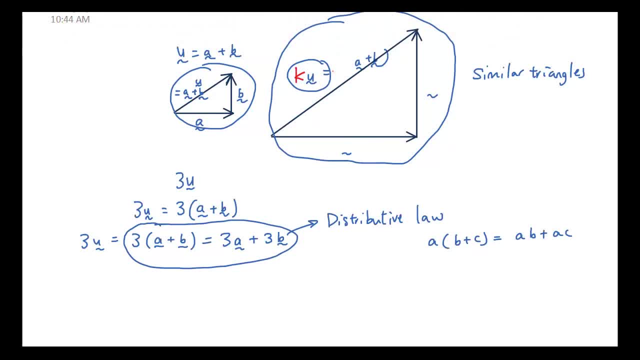 So I could write k. okay, I could write k: Doesn't matter, But scale factor. I multiply this triangle by this distributive law will work. Okay. so let's write a distributive law properly: k, bracket a plus b.